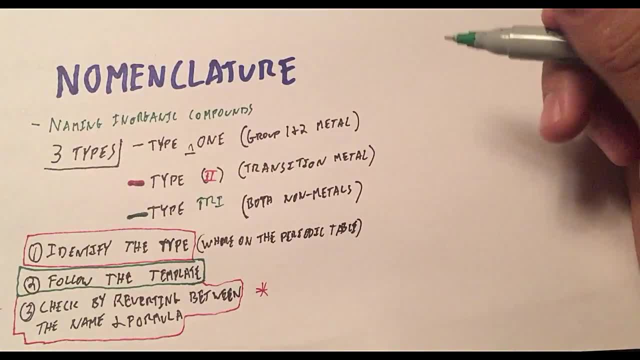 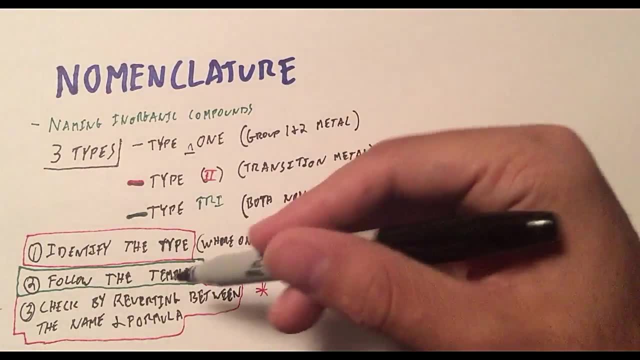 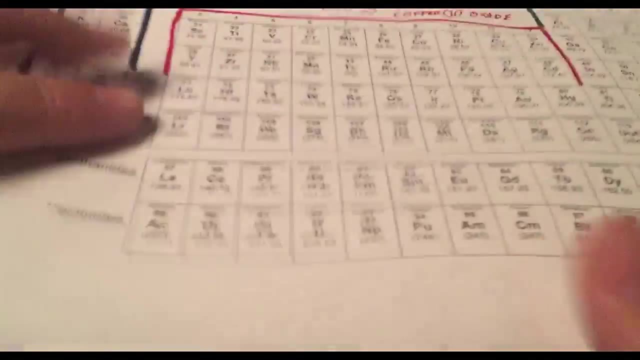 prefixes like di, tri and tetra and things like that to do that naming. So I'm just going to go ahead and show you the formula or the template for naming each one of these compounds. okay, So when you have type 1 or none that involves a group 1 or 2 metal, Look here on our periodic. 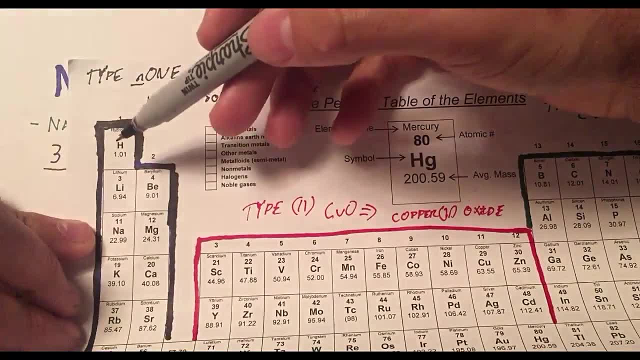 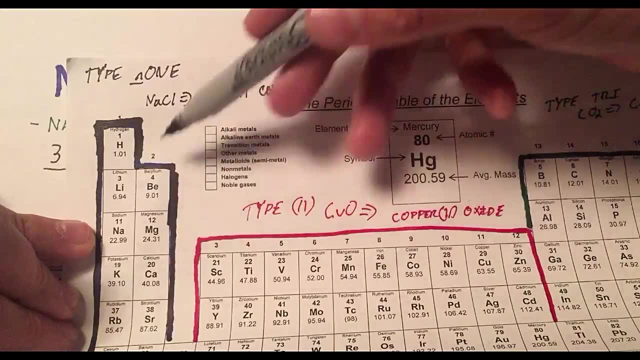 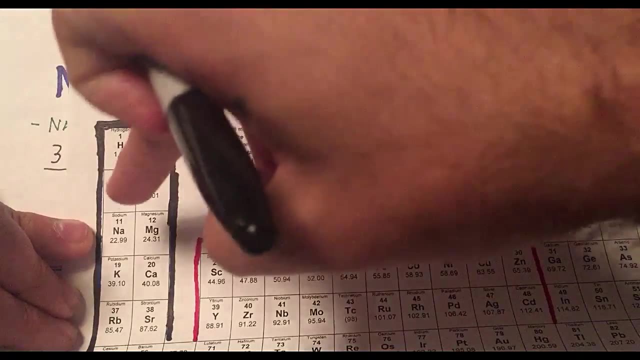 table. that means we're dealing with anything in this first group right here. So hydrogen, lithium, sodium, beryllium, magnesium, any of these. Now we know that these are 1 plus and 2 plus charge, And all of these compounds are going to be between a metal here in these two groups. 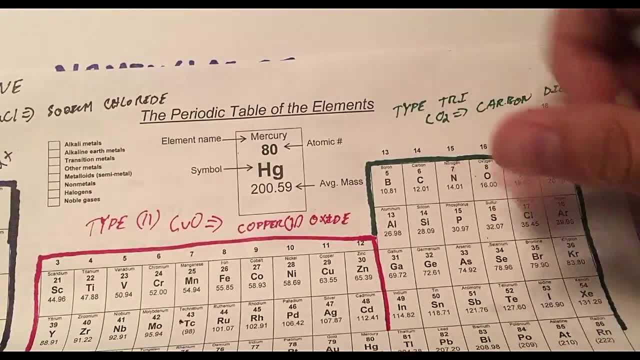 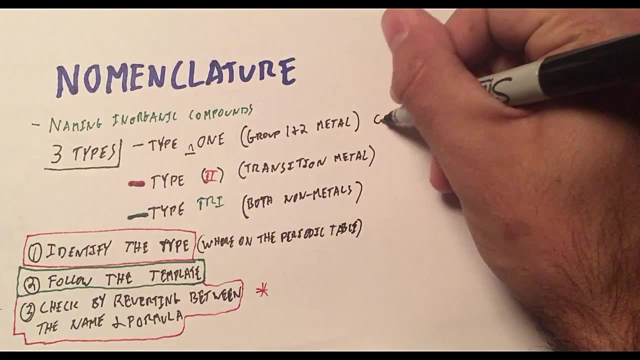 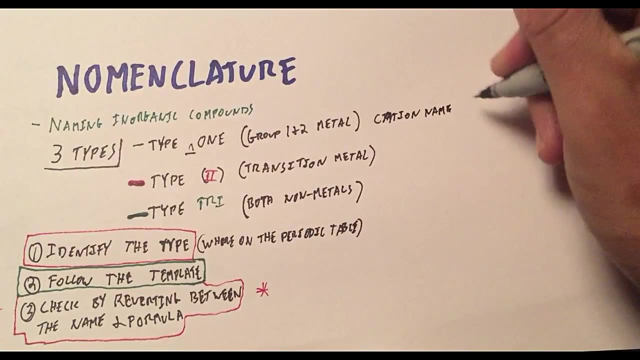 and then a non-metal over here in this group. So we're going to be dealing with any of these compounds in the p block, okay, So let's do a quick example or show the template. actually, We have the cation name, We have space, and then we put the anion and we end it with the ending "-ide". 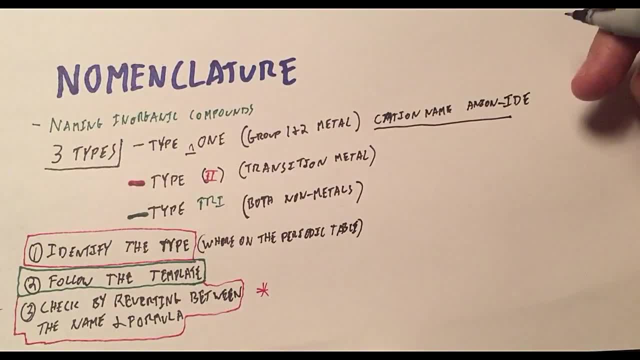 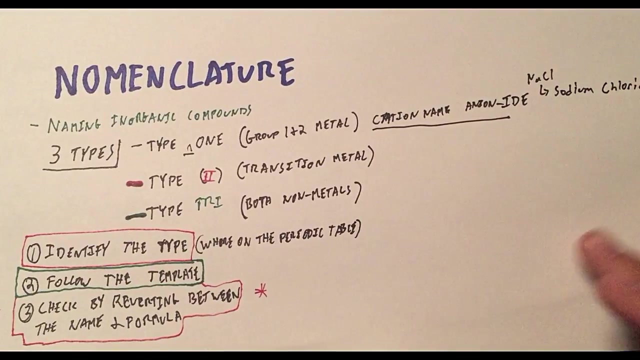 Okay, So, for example- so this is clear- something like Cl would be sodium, and that's the cation name, the positively charged species that we're dealing with. So sodium positive plus 1, sodium chloride. That's all That's it. That's how easy it is when 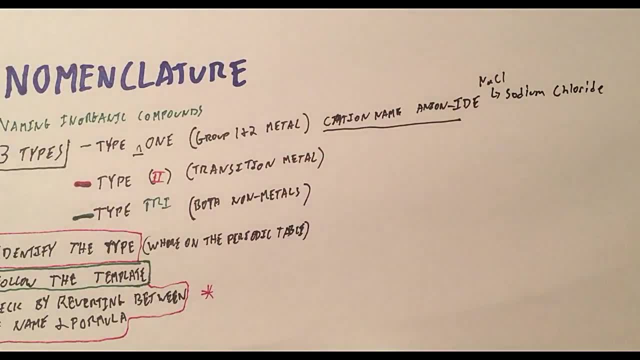 it's type 1.. And that's why I call it type none, because there's nothing you have to do, And the idea there is that anything that's in group 1 or 2, you know the charge, It's plus 1, plus 2.. 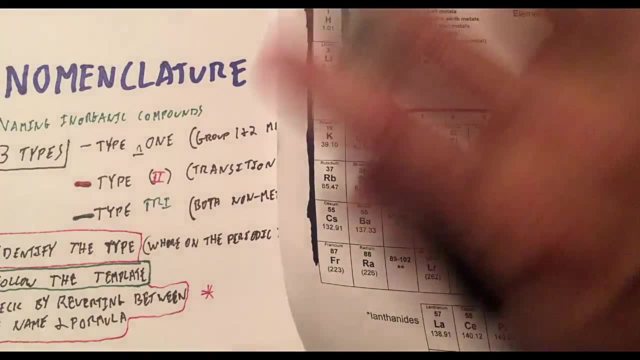 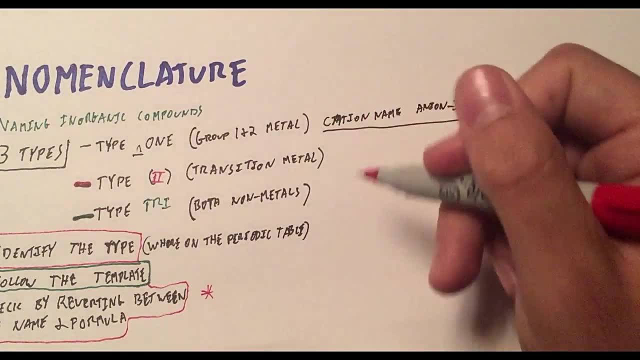 So, therefore, you don't have to indicate to whoever's reading the name that there's anything else going on. It's just 1, 2.. Okay, Let's go ahead and do type 2, which involves a transition metal. This is where we're going to have the cation name again, So I'm just going to put a space for. 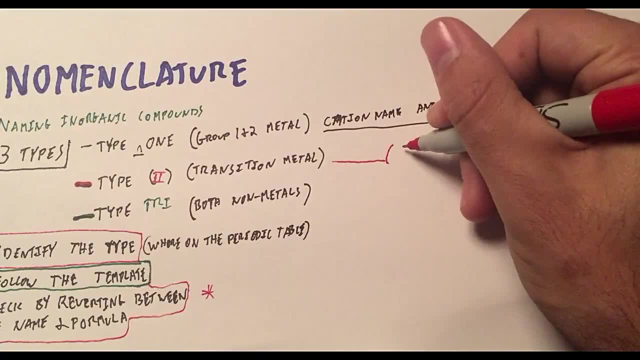 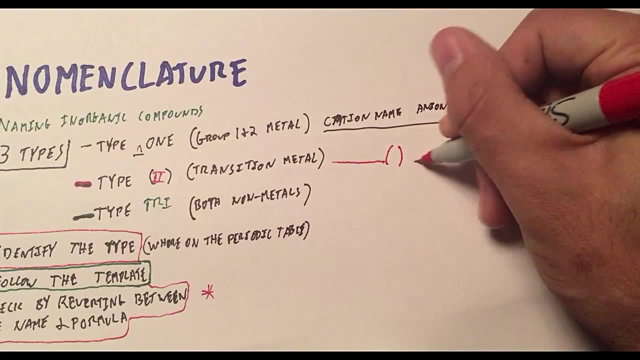 that name. okay, Then you're going to have roman numerals without a space. okay, So they're going to be right on that name. Then you have a space and the anion name that you're going to end in "-ide again" okay, Okay. So an example of this would be something like this: So you're going to have a. 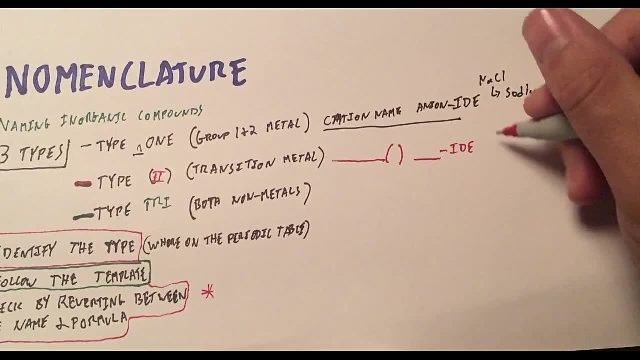 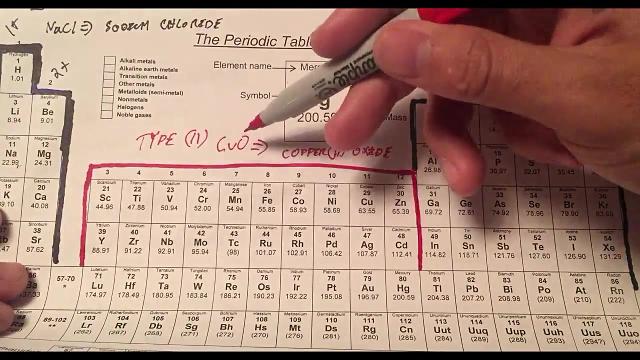 something like: let's see copper oxide. okay, Now to do this name, I have to consider what the charge on copper is, because it's a type 2 naming, And here I see type 2 copper. What this means is: 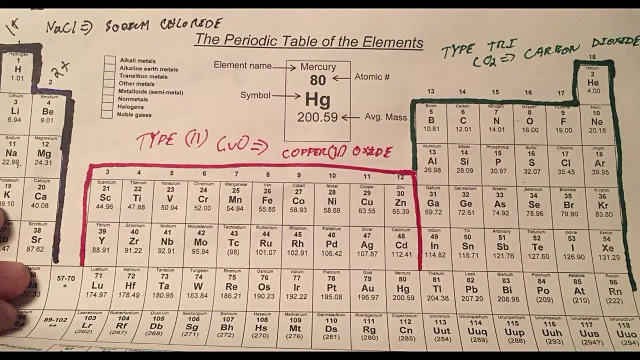 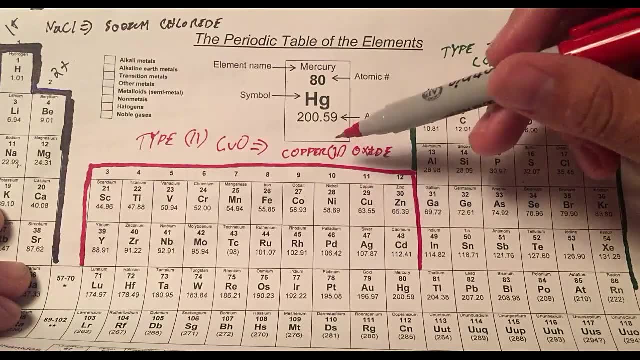 that we do not know the charge on copper. Copper can take different oxidation states. That's why it has different colors. It can form hydroxides and things like that. But essentially we have to recognize that copper doesn't have a distinct charge, so we have to indicate it. 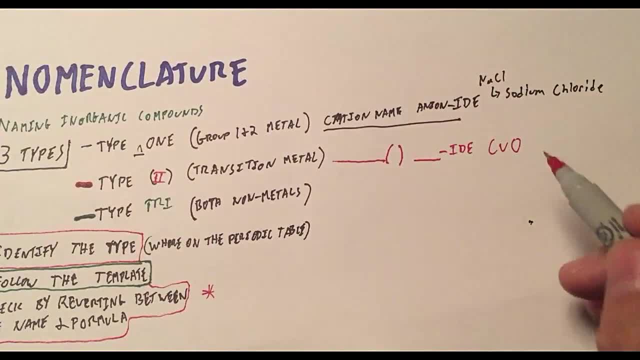 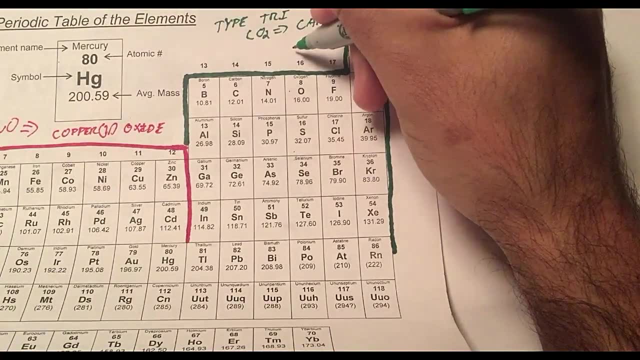 to whoever's reading the name what it is. Well, if it's CuO, I know that oxygen has a charge of 2- right, Because it always does well when you're dealing with this type of naming. So that's. 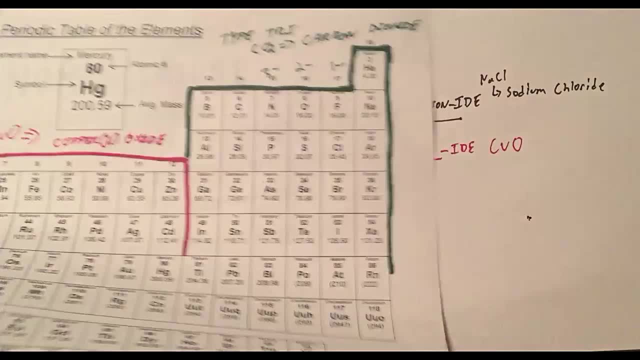 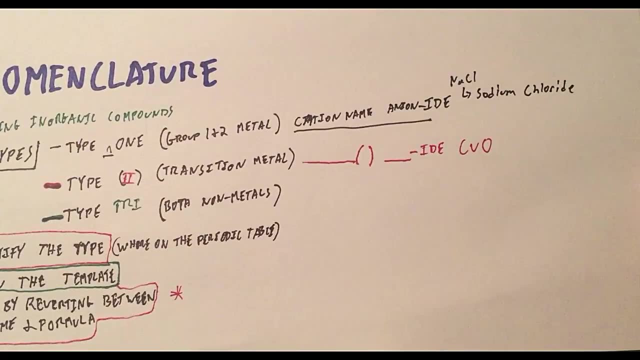 2-. right, Let's go ahead and put these in now. If oxygen has a charge of 2- and there's only one copper here, then this copper must therefore have a charge of 2+, right, Because it's. 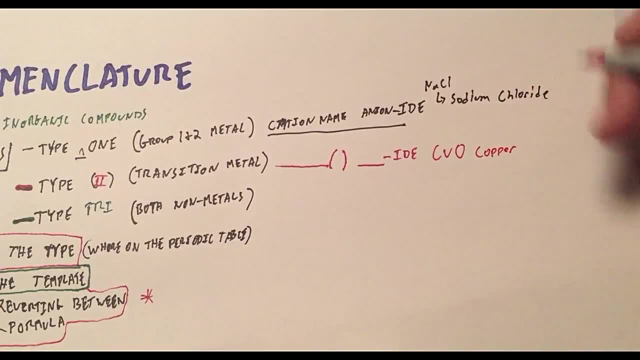 got to balance out to zero. So that gives us copper oxide. That 2 means that copper is plus 2, has a 2-plus charge. That's all it means. It doesn't mean that there are two coppers, It just. 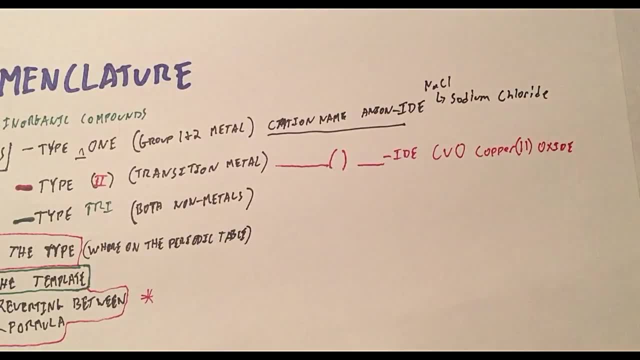 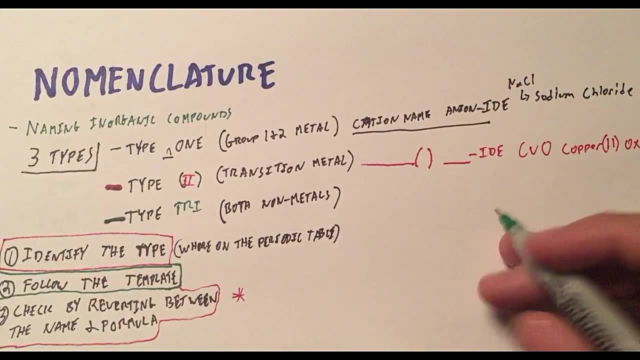 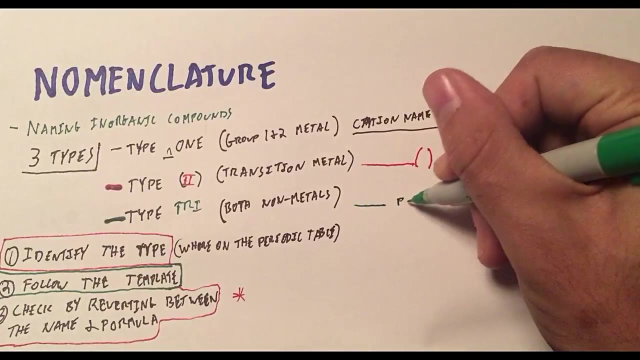 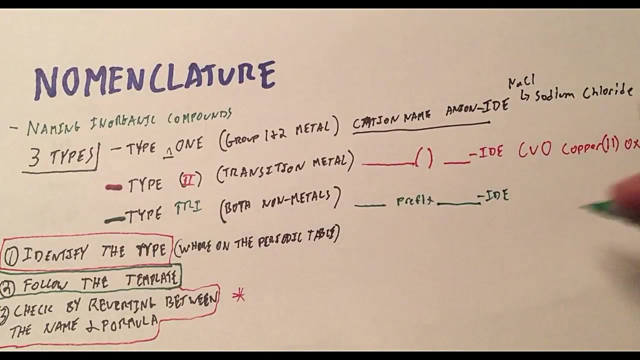 means that it has a 2-plus charge. Okay, we'll do some more examples of that. Let's go ahead and look at carbon dioxide: okay, And this is where you're going to have name and then prefix and then name with I-D-E as the ending. okay, So let's go ahead and just do CuO right And you. 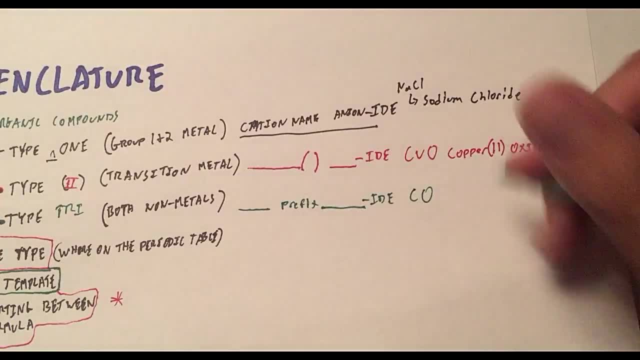 guys have all heard of this. I have copper. That's my first name, okay? Have I been saying copper this whole time? Carbon, carbon monoxide, right? So we have carbon monoxide. That's the bottom. Let's go ahead and put carbon monoxide. Mono is the prefix for one. There's only one. 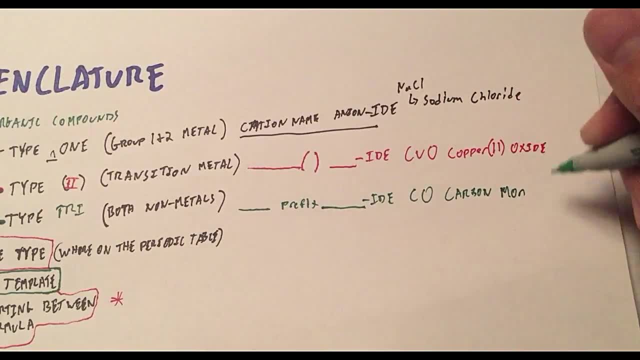 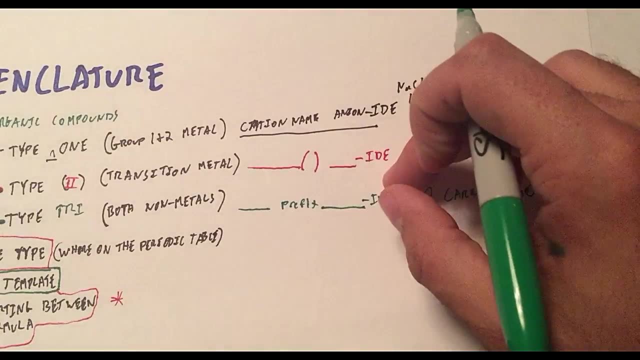 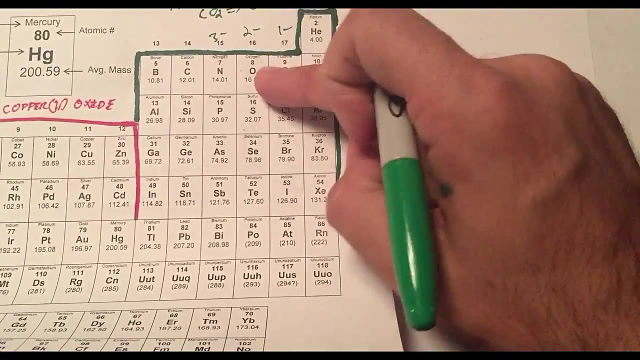 oxygen there. therefore it's carbon monoxide. okay, That's all. Now you know it's type tri when you have to deal with two elements that are both in this group, Carbon and oxygen are both here. okay, So to refresh this real quick: type one are the first type. type none are the first. 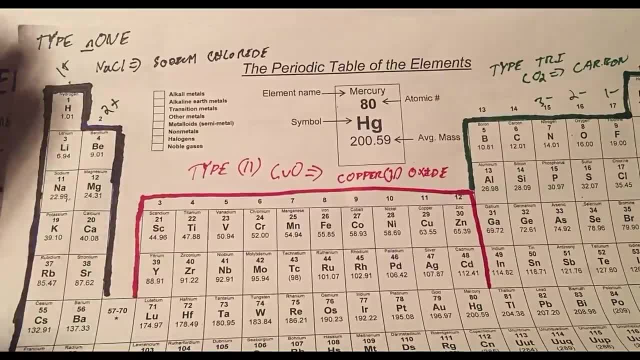 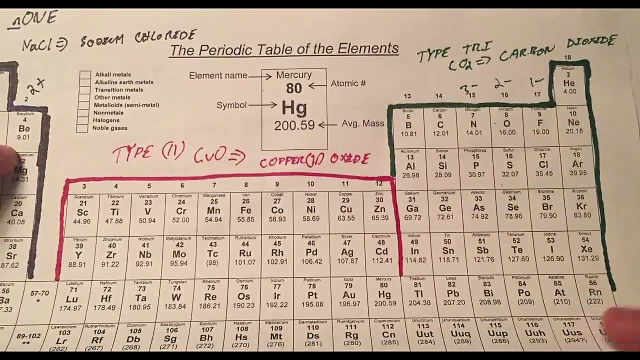 one, We don't have to use any Roman numerals, any prefix, anything, So it's type none, okay, And that's when you're dealing with something from here, with something from here, okay. Then when you have type two, you don't know the charge, So you got to use the Roman numerals, something from. 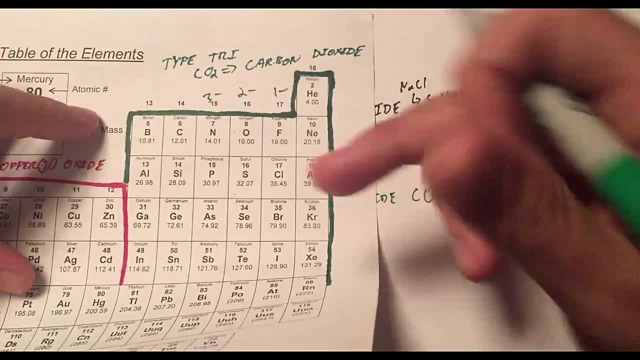 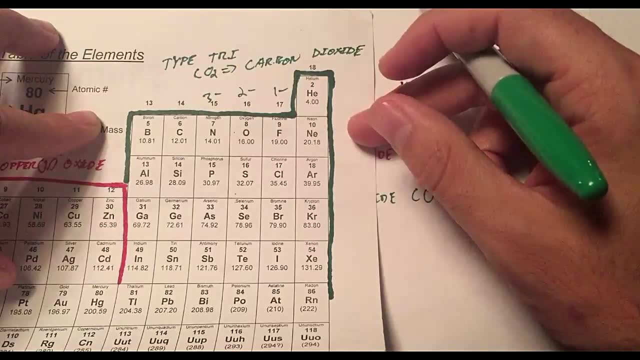 here with something from here. Type tri, you know their charges. However, you're dealing with metal or two nonmetals bonding together, so the charges are changing or the oxidation states are changing, and that's a whole other topic. But that means you're dealing with something from here with. 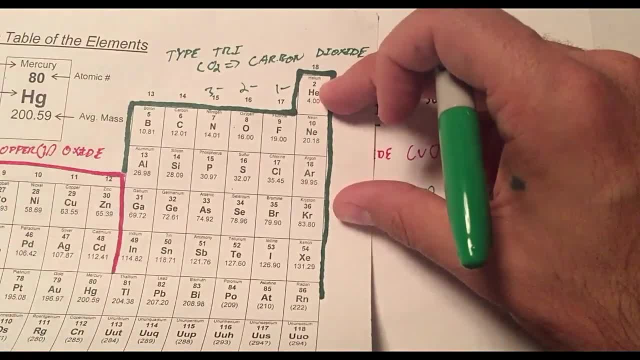 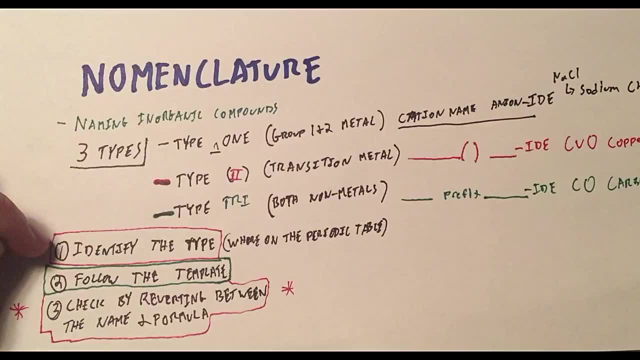 carbon dioxide, something of that sort. okay, Let's go ahead and just summarize this right here. The first thing you're going to do is you identify the type you're dealing with. It's not that important that you know that copper oxide is type two naming. That's not really what I mean by that. 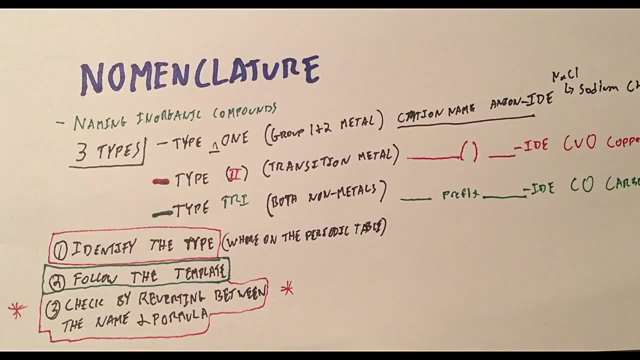 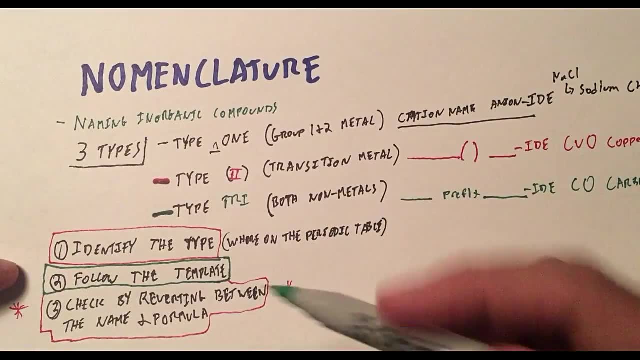 What I mean by that is just understand. am I going to use Roman numerals or not, Am I going to use prefixes or not? Follow the template and that's using the space and the ide, okay, the ending and how that's going to work out for you, And then go back and forth between the name and the formula. 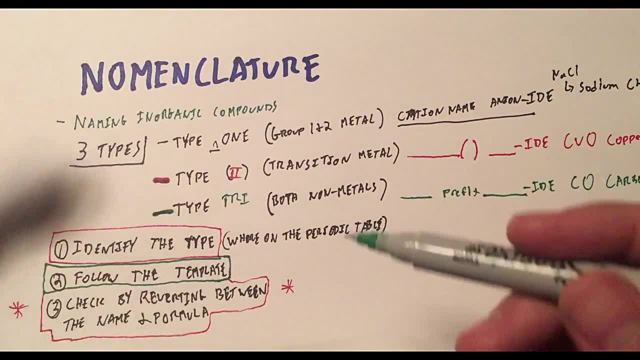 if you can get the name from the formula, you're good. or you can get the formula from the name, all right. Let's go ahead and do a couple examples.